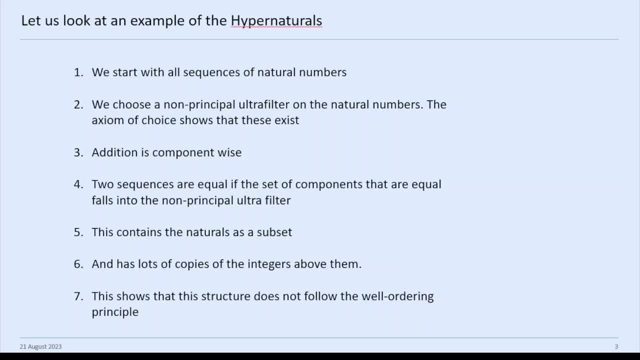 natural numbers and the axiom of choice shows that these exist. Addition is component wise And two sequences are equal if the set of components that are equal falls into the non-principle ultra filter. So basically, they're equal if almost all of their components are equal. 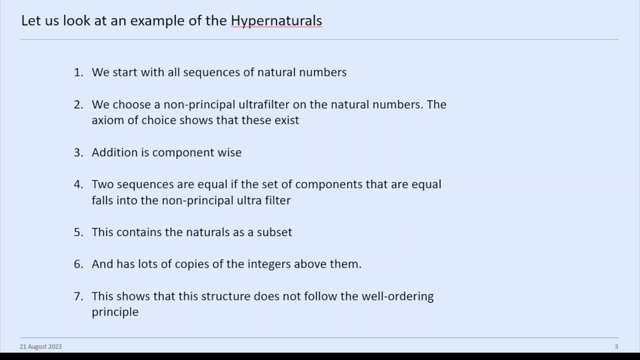 where almost all is defined as being a member of the non-principle ultra filter. So this contains the natural numbers as a subset which will show, and it has a lot of the copies of the integers above it And we can see why the structure does not follow the well-ordering. 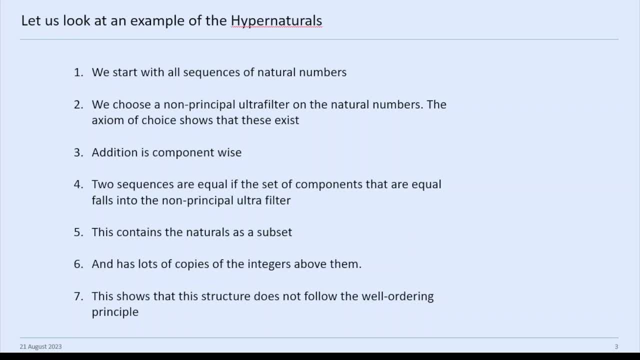 because if we choose a bunch of elements of the integers, that set, if it's an infinite set, may not have a least element. And also induction is not able to jump from the naturals up to these copies of the integers. Whereas induction can run through all the naturals, it can't jump into the. 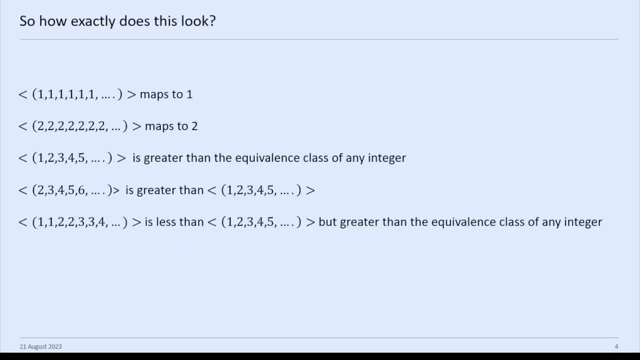 integer sets. Okay, So how is how does this look? So basically, you've got All of the ones maps to one, So the equivalence class of the string of all of the ones maps to one. So, for instance, in that equivalent class. 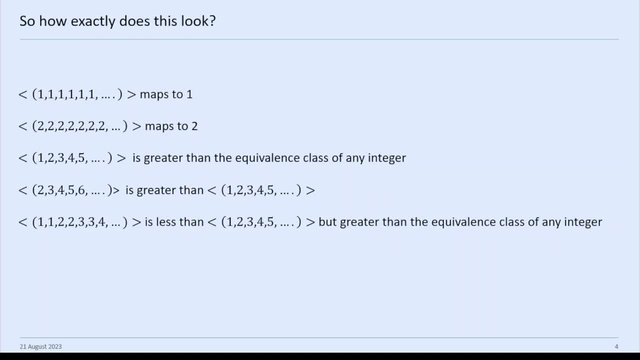 you could have something that goes to 1,1,1,1,1,1,1,1,. that's fine. That just is still mapping to one. The string, the equivalence class of the string of all the twos maps to two. 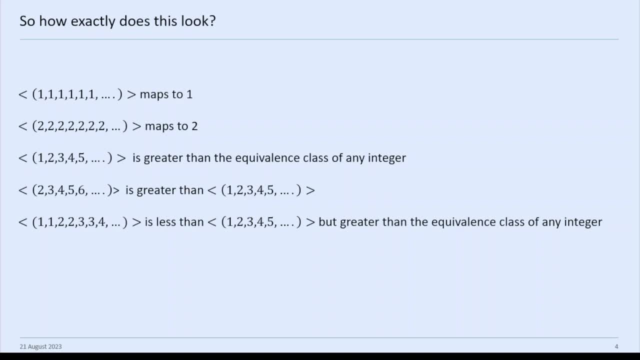 The equivalence class of the string of all the ends maps to n, But then 1,, 2,, 3,, 4,, 5,, 6,, 7 is greater than the equivalence class of any integer because for almost all of the components they will be greater than n for any n. 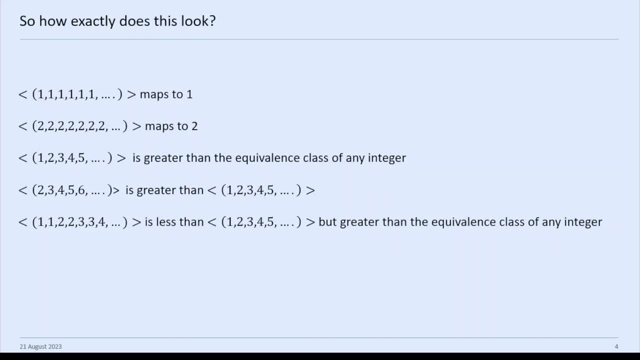 So this is the. this is a sort of plays the role of something that's bigger than all the integers, And then 2,, 3,, 4,, 5, 6 is bigger than 1,, 2,, 3,, 4,, 5.. 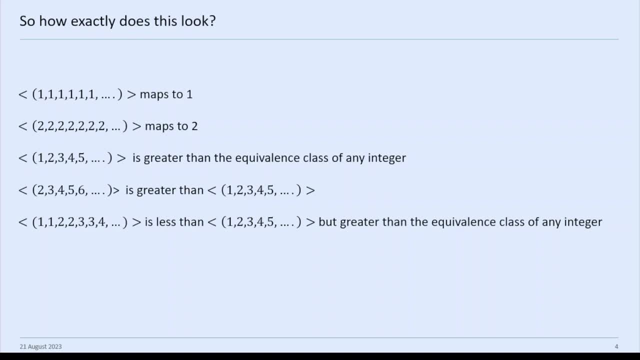 And 1, 1, 2, 2, 3, 3, 4, 4 is less than 1, 2, 3, 4, 5.. And 1, 1, 1, 1, 1, 2, 2, 2 is less than 1, 1, 2, 2, 3, 3.. 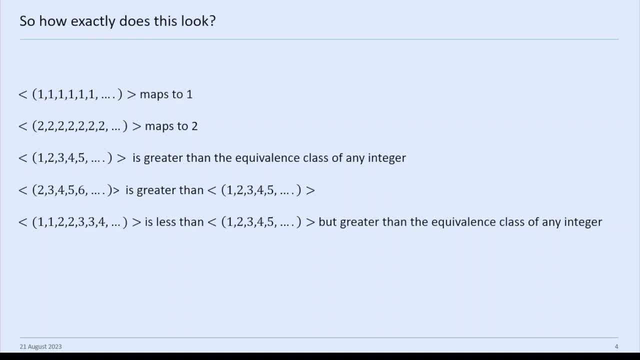 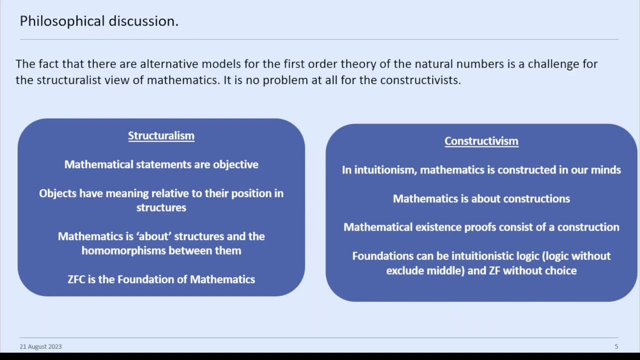 And if you think about this for a bit, we can see how rich the structure is and how many options there are and how many kind of equivalence classes could be built. So non-standard models of first order arithmetic do raise some philosophical questions And I think it's a kind of challenge for the structuralist view of mathematics, and we'll see why. 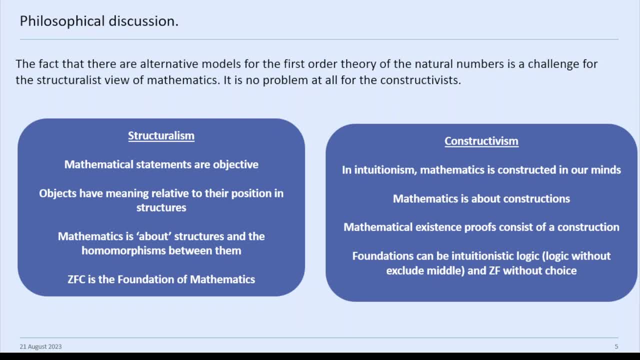 But before we get into that, we're going to just define structuralism and constructivism. So For structuralism, in a structuralist view of mathematics, mathematical statements are objective, Objects have meaning relative to their position in the structure. So the whole content of the number 3 is its relationships with 1, 2,, 4,, 5, 8, etc. 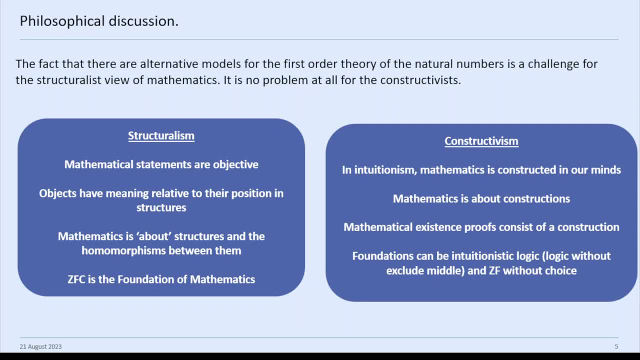 If you want to understand 3, you need to understand its place in the naturals. Mathematics is about structures and the homomorphisms between them and the structure-preserving mappings. And the structure-preserving mappings is about structures and the homomorphisms between them. 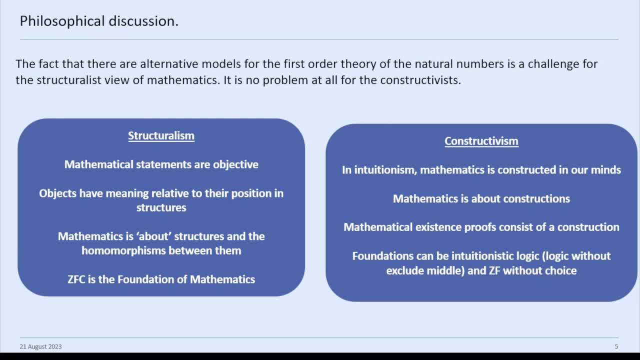 And ZFC. ZF set theory with choice is basically the foundation of mathematics under a structuralist view of the world, Although some want to use category theory and I have some sympathy for that view. But most people think of it as ZFC. 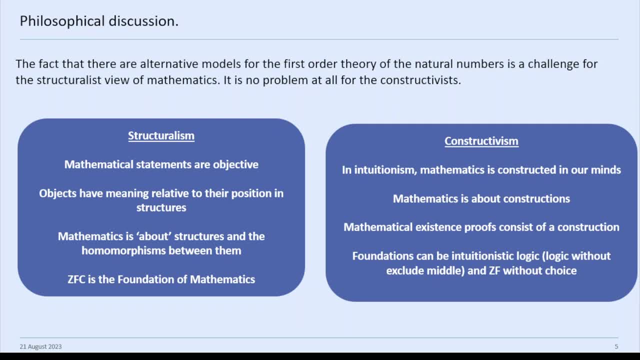 Constructivism. So intuitionism is a certain brand of constructivism in which mathematics is built in our own minds and so it's subjective, not objective. But there are versions of constructivism that are not intuitionism. Mathematics is kind of about constructions. 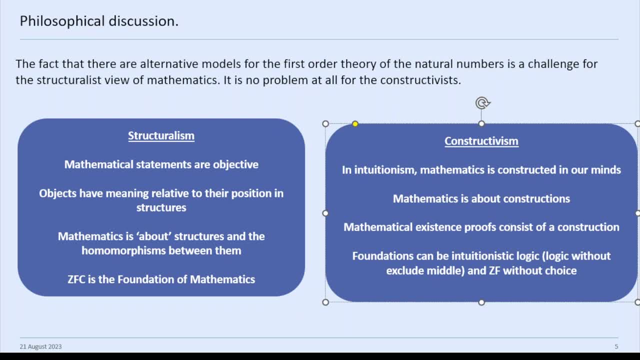 Actually, if I'm going to put about in quotes on the left, I'm going to put about in quotes on the right. Mathematical existent proofs consist of a construction of the thing that you're showing exists. So the kind of existential qualifier in mathematics corresponds to the fact that you can make a construction. 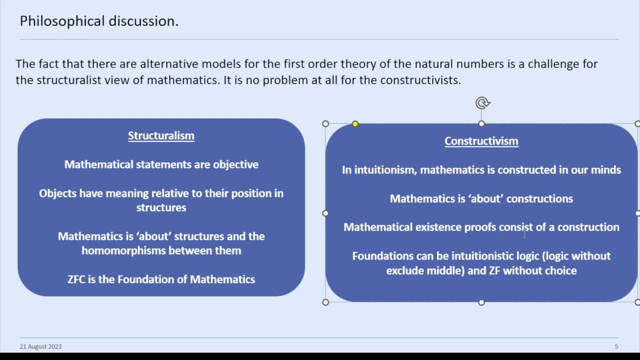 And that kind of means that you can't have excluded middle, because you can have a situation where you can't build something, but you can't constructively show it can't be built. So the foundation could be intuitionistic logic, which is basic logic without excluded middle. 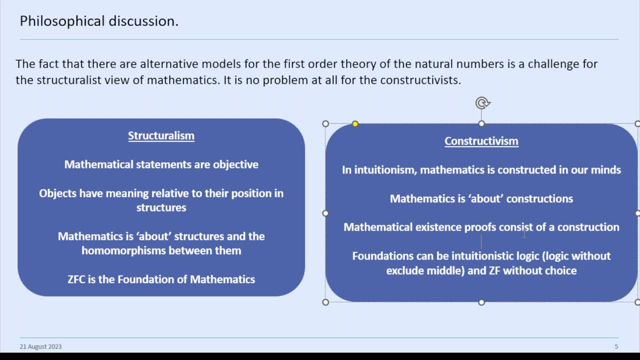 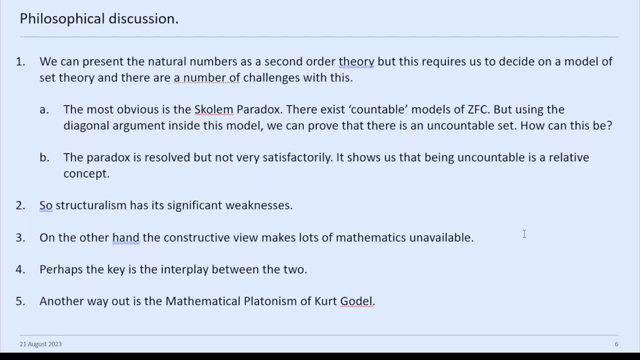 Or some constructivists want to use ZF without choice. I think there's a feeling that choice is quite non constructive. um, so that's the kind of difference between those two broad methods of thinking. and so having alternative models of first order arithmetic is a problem, because 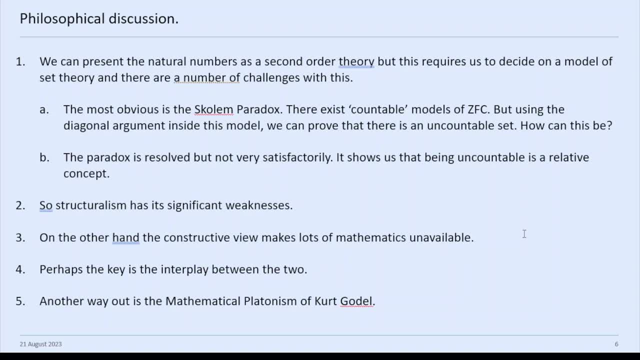 i might worry that i don't have the same model in my head as you do, and the constructivist would be less worried about this. but if we, if we're structuralists, we might care that we might have different models in our head. if i just describe it to you in terms, 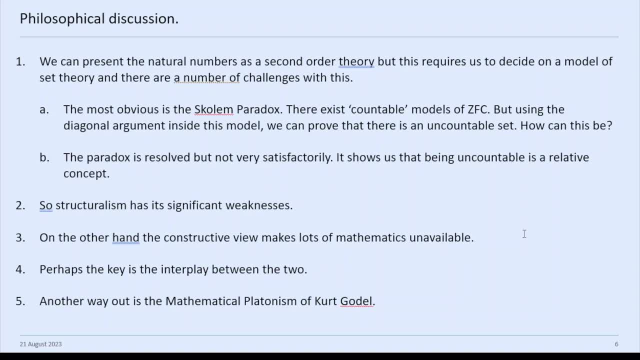 of the first order sentences. how do you, how do we know that we've got the same model in our heads. so one way around this is to present it as present the natural numbers, as a second order theory. so, for instance, that would mean that we do have induction, because induction is a kind of second. 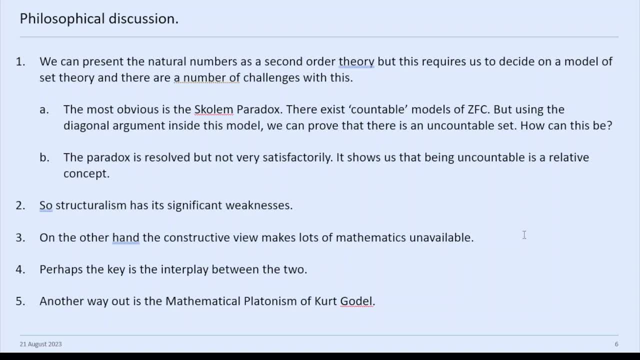 order statement because it's about sets, isn't it? and the well-ordering principle is about sets. so the problem with this, actually, or a problem with this, is scott, the scollum paradox, which basically shows there are countable models of zfc. they look countable to us, but if we use the 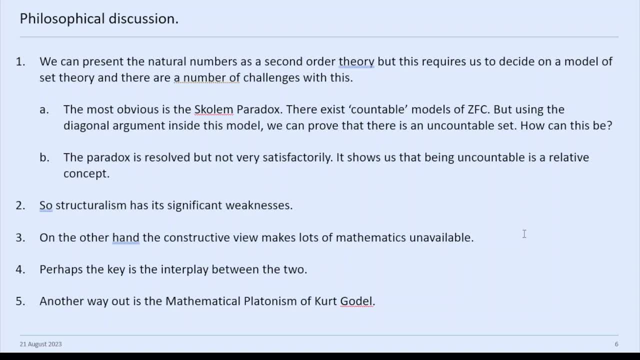 diagonal argument inside the model, we can find an uncountable set within the in the model. so how can it be there's an uncountable set with an accountable model? well, the reason is because this countable model is really small, so a bunch of mappings are missing and uncountability is about 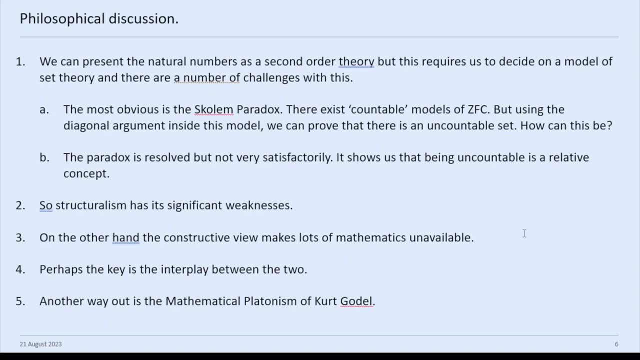 the non-existence of a mapping, so we can prove that a set is uncountable within the model because that mapping is missing. but this is kind of a resolution, but it's not entirely satisfactory because it shows that being uncountable is a relative concept. you're kind of uncountable from within the model, but 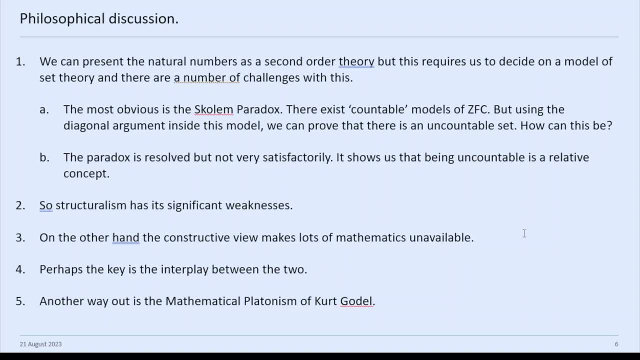 countable when looking in from outside, which is odd. so there are some real complexities or even weaknesses around structuralism. on the other hand, the constructive view does make a lot of mathematics unavailable, because it means you can't prove um, you can't do proof by contradiction or